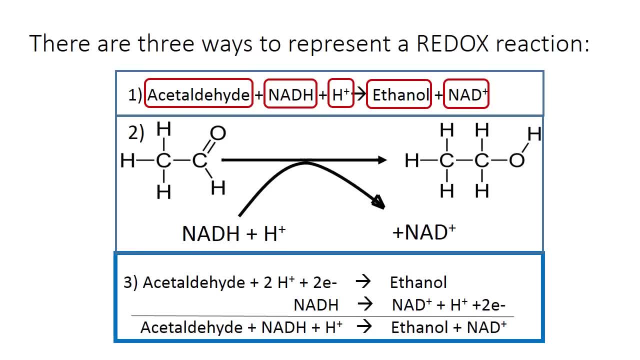 into two half-reactions. The top reaction here is the reduction 1,2- 1 and the bottom reaction is the oxidation 1,2- 1.. We know this because of where the electrons arrange in the half-reaction. If we form ethanol, we need to add 2'0 electrons to acetoaldehyde. then 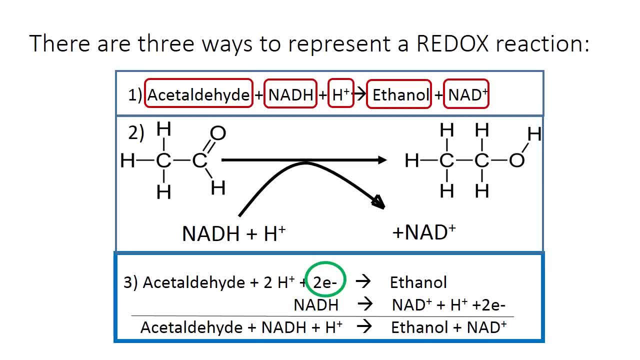 we know that ethanol is the product of inventions of 2 intelligence onto acetoaldehyde. Also, we know that Reduction is gain of electrons, partrosoo oxidation, half reaction. If we look at the before and after, if we removed two electrons from NADH, we produce NAD+. Loss of electrons is oxidation. 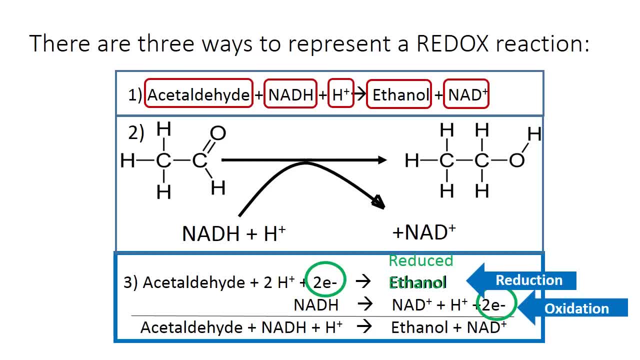 Therefore, in this reaction, we can say that ethanol is the reduced form, that acetyl aldehyde is the oxidized form of the carbon compound. NADH is the reduced form and NAD plus is the oxidized form of this compound. NADH is really. 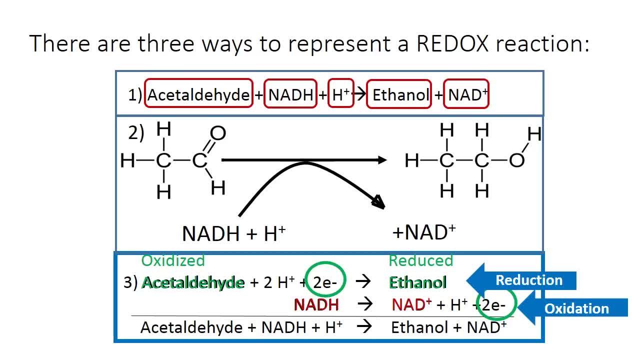 important in metabolism. You're going to see this compound over and over again. This is an electron carrier. It moves electrons from one place to another in the cell. So when you see it as a reactant or a product of a reaction, you automatically know that it is a redox reaction. If we didn't have the half 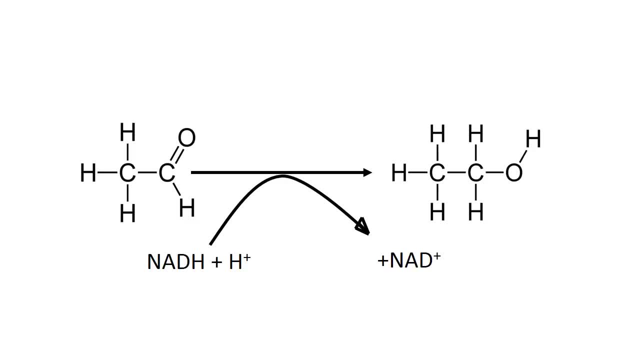 reactions, then we could take a look at the structure of the compounds to determine if they were oxidized or reduced. In biology we deal with a lot of metabolic reactions that oxidize or reduce carbon compounds. In this example we can see that acetyl aldehyde has four carbon-hydrogen. 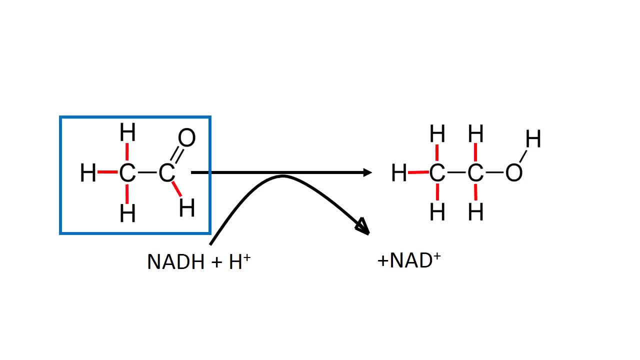 bonds compared to that of ethanol that has five carbon-hydrogen bonds. We know that electrons can move with hydrogen atoms. So when we compare these two compounds, the one here with more carbon-hydrogen bonds is more reduced than the compound with less carbon-hydrogen bonds. But why did this? 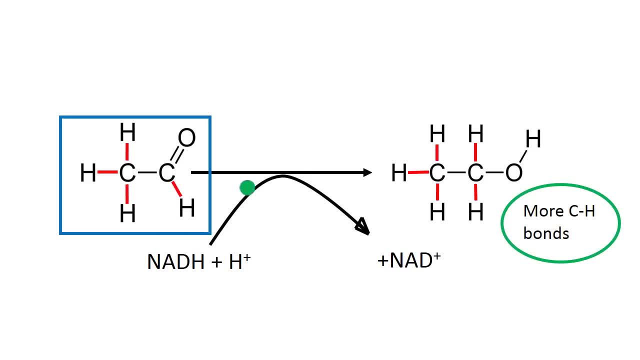 happen? Why did electrons move from NADH onto acetyl aldehyde to form ethanol? Why did electrons move from NADH onto acetyl aldehyde to form ethanol? This is not something that you're going to need to memorize for every single. 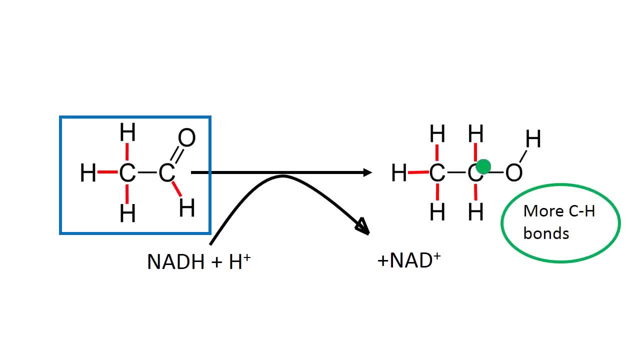 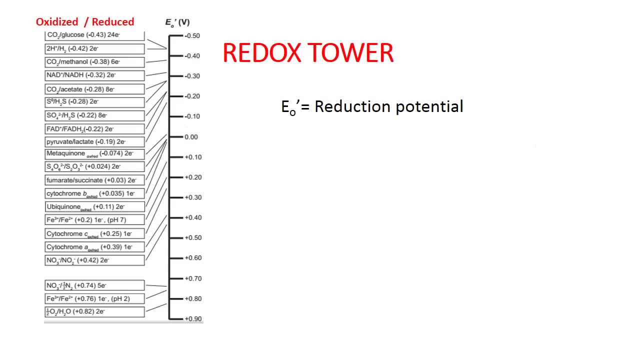 metabolic reaction. There is a tool called a redox tower that we can use to predict the movement of electrons in biological reactions. Here's the basic structure of a redox tower. We have a list here of half reactions and their E-value. This value is the reduction potential, which is the likeliness of a. 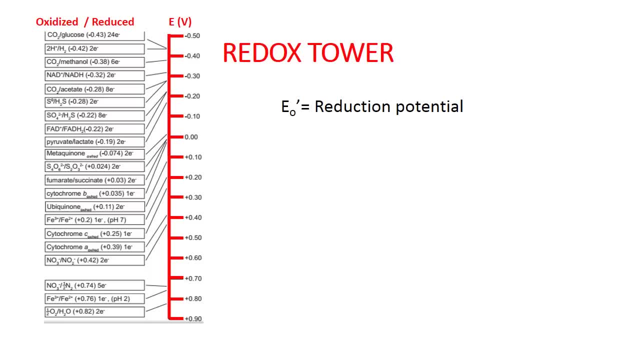 compound to gain electrons. The organization of the tower should show positive E-values at the bottom, with negative E-values at the top. This means that the compounds at the bottom of the tower are more likely to gain electrons when you compare one of these compounds to one at the top of the tower. 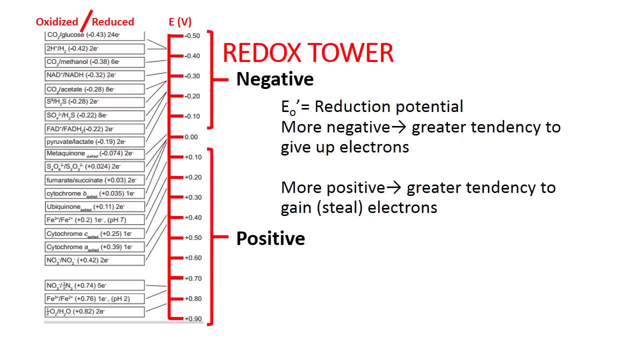 You may also notice a slash on each line of the tower. On the left-hand side of the slash is the oxidized form of the compound. The right-hand side is the reduced form of the compound. Let's take a closer look at the electrons moving from one compound to. 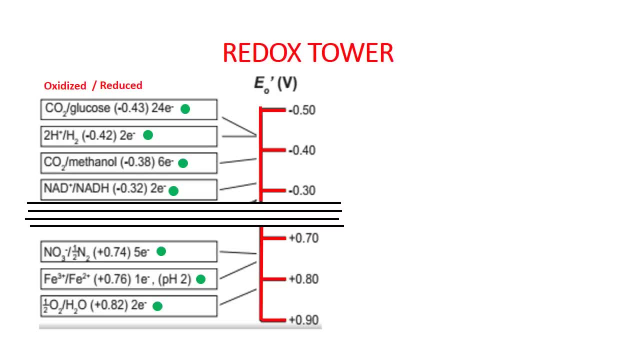 another using the redox tower. Let's combine the two half reactions shown here, hydrogen gas and NAD+. When we combine two half reactions using the redox tower, we can answer several questions about the reaction. We can ask which compound is the electron donor and which is the electron acceptor Using just the 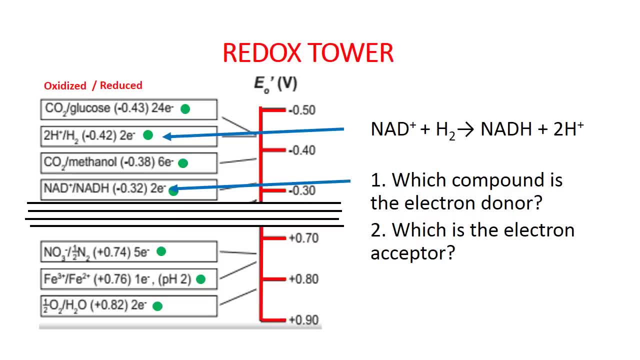 information in the tower, we can see that the NAD half reaction sits below hydrogen gas on the tower. Compounds that sit lower on the tower are more likely to gain electrons. Therefore, the electron donor needs to be either hydrogen gas or the protons. From here you look at either side of the slash, The oxidized form, and 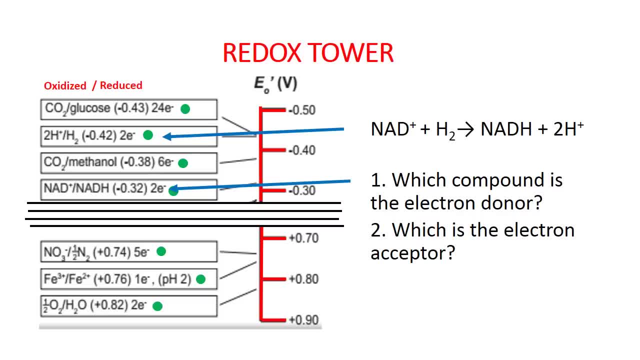 the reduced form of this compound. The reduced form has electrons. The oxidized form does not. Therefore, hydrogen gas will be the electron donor. This electron will fall down the tower and reduce NAD plus to form NADH. Let's look at one more reaction. This is an equation often used to represent the 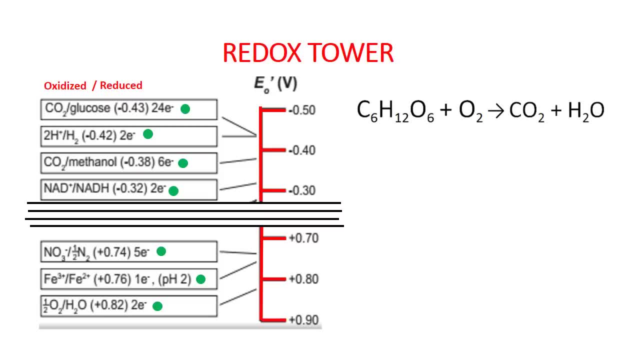 many reactions involved in central metabolism. First let's find our two half reactions. Glucose is here at the top and oxygen is here at the bottom of this tower. Let's ask our questions again: Which compound is the electron donor and which is the electron acceptor? The glucose half reaction is above the 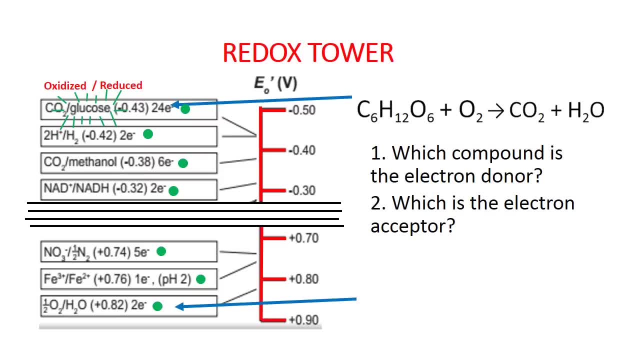 oxygen half reaction. Therefore the reduced compound of the top half reaction will act as our electron donor. So when oxygen here accepts electrons from glucose, which oxygen wants to do, not just because it's at the bottom of the tower but also because it is below the glucose half, 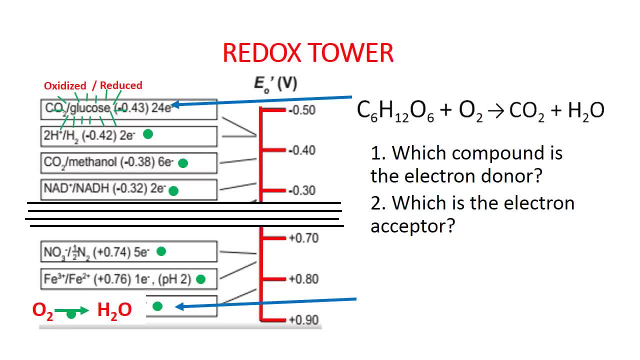 reaction, it will become reduced forming water.